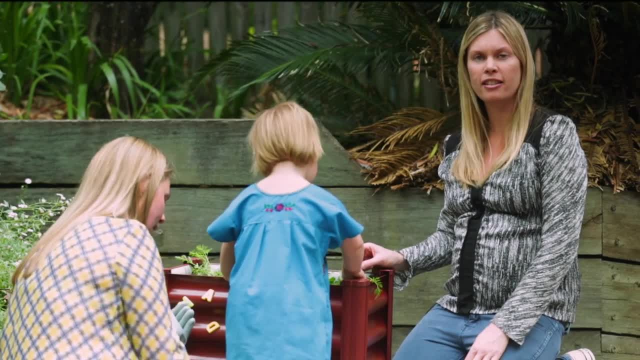 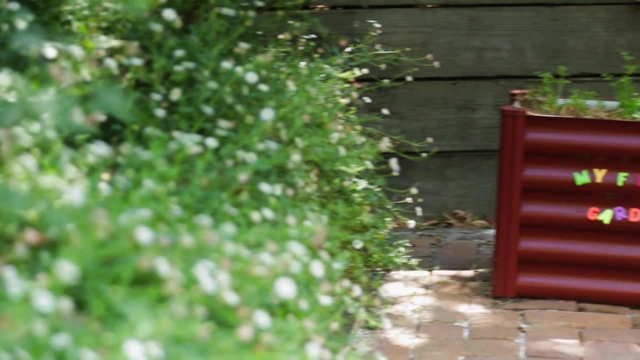 My sister and I wanted a way for our little ones to have more time outside and to learn more about nature and the environment, And that's how the idea of My First Garden was born. My First Garden is a rewarding hands-on activity for growing minds. With My First 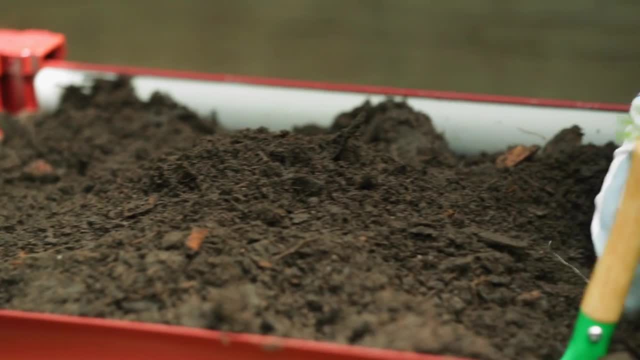 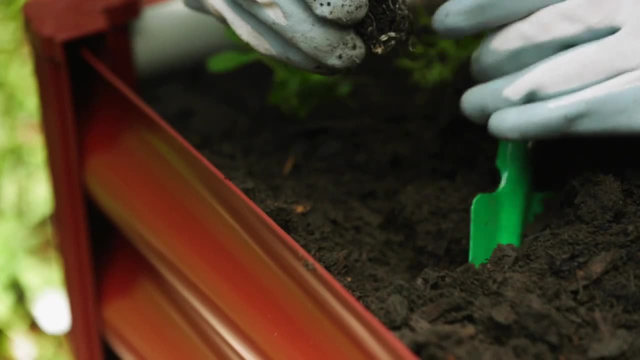 Garden. children will learn important lessons as they care for plants, develop fine motor skills and are encouraged to make healthy food choices, all while being active. Plus, it's a fun outdoor activity that the whole family can enjoy. I want to show you how easy. 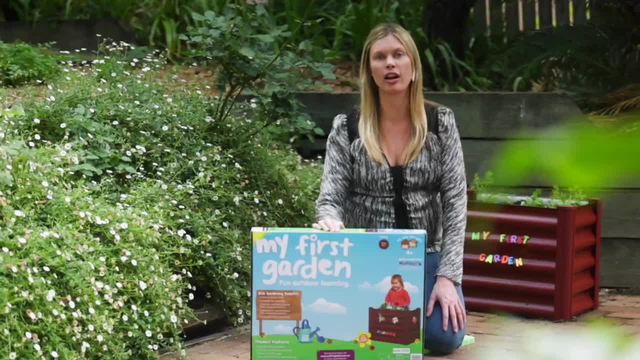 it is to assemble your My First Garden and start planting with your child While My First Garden works. it's also a great way for children to learn more about nature and the environment. My First Garden is a rewarding hands-on activity for growing minds, With My First Garden children. 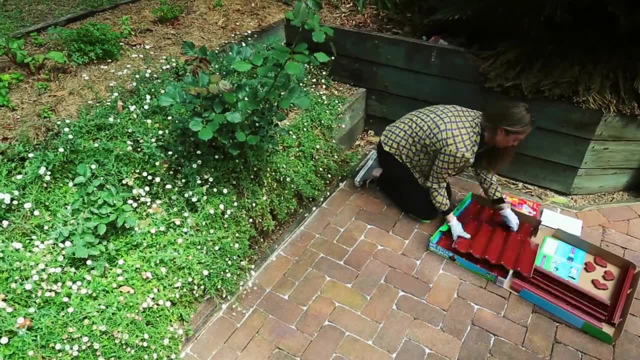 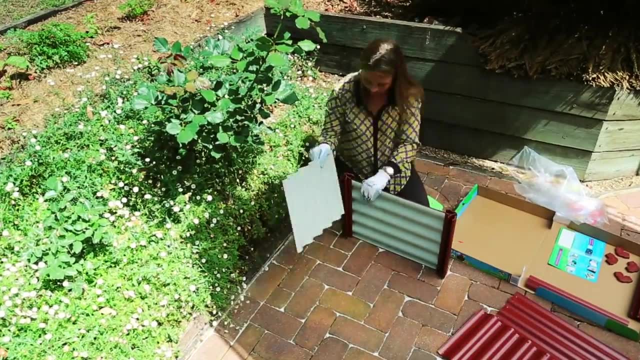 is designed for children aged four and up. Your garden bed should not be constructed by any persons under the age of 14.. When the garden bed is assembled, the exposed edges of your garden bed are rolled for your children's safety. Some of the side edges that won't 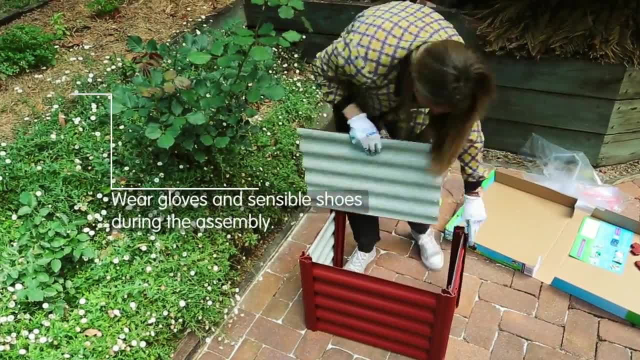 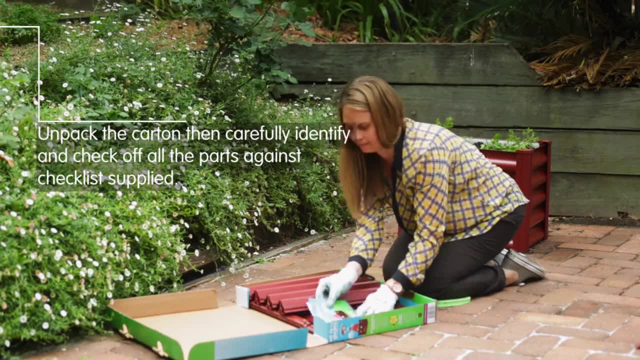 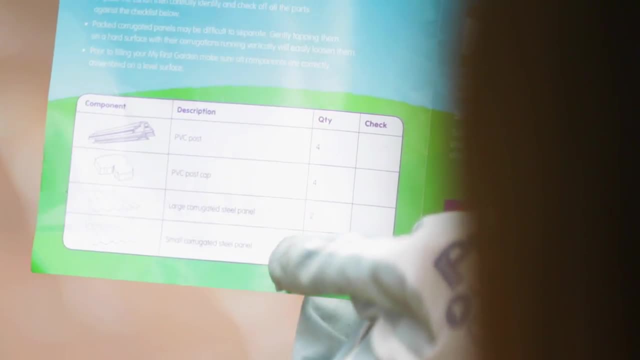 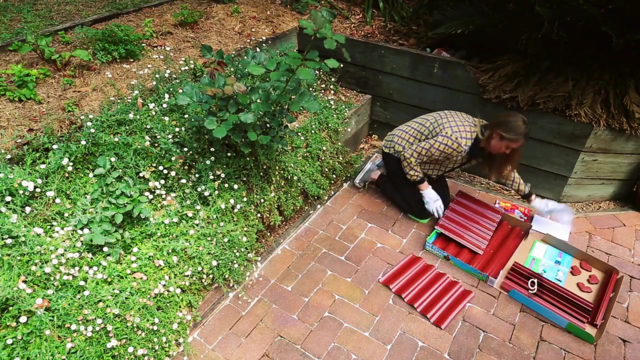 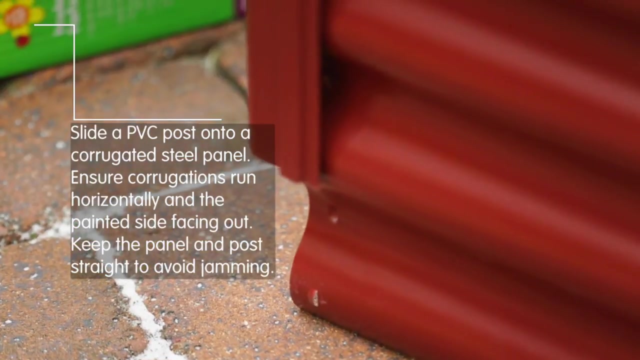 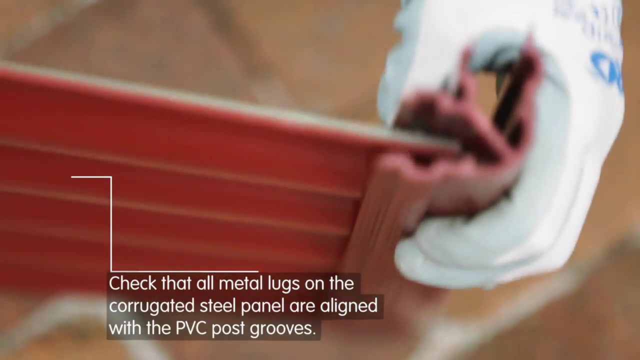 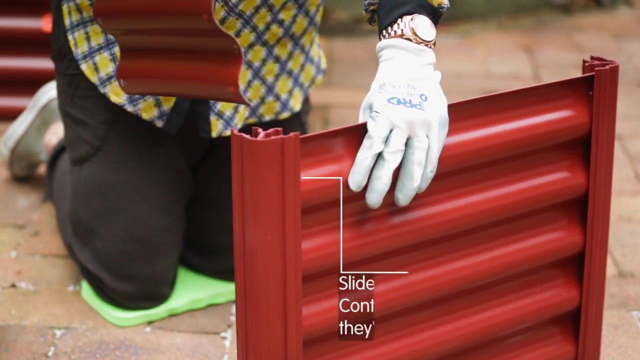 be exposed may be sharp, so we recommend wearing gloves during the assembly. Sensible shoes are also recommended. My First Garden's home is right outside My First Garden. We are a family of gardeners from my own home, My First Garden, has been living with my children for almost ten years. All of my children, including 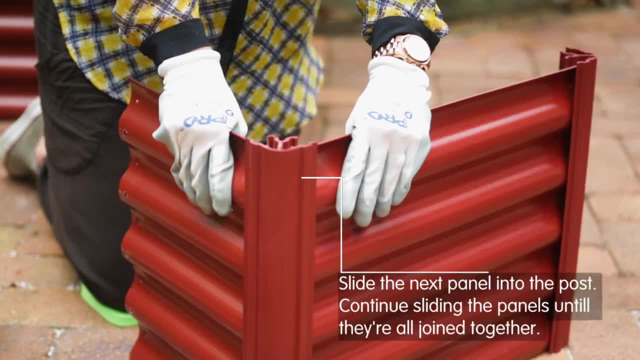 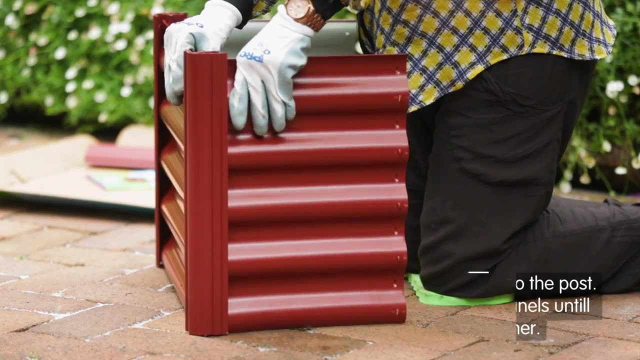 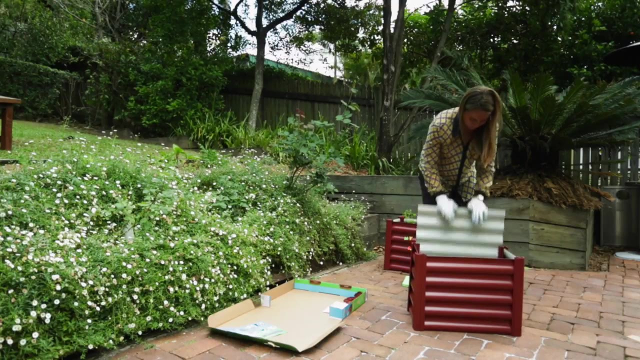 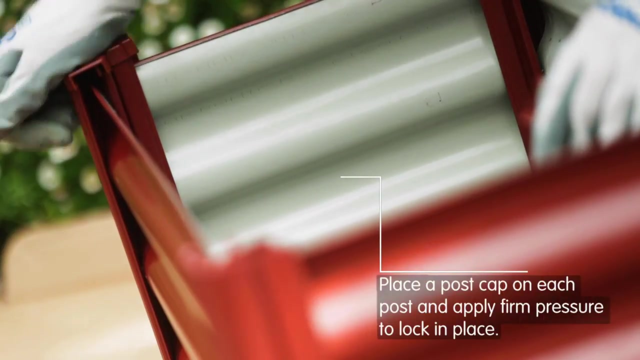 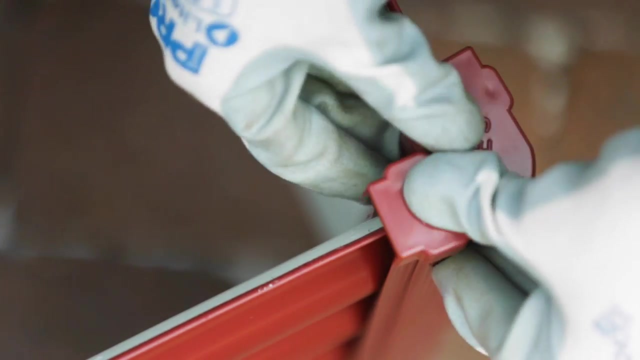 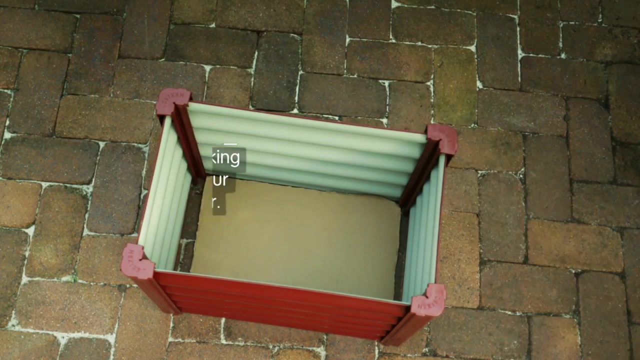 Thank you. Now that an adult has assembled your My First Garden, we can get our little helpers to come and help plant and decorate our garden bed. If your kids are like mine, they will love decorating their garden with the colourful magnets that come in each box. 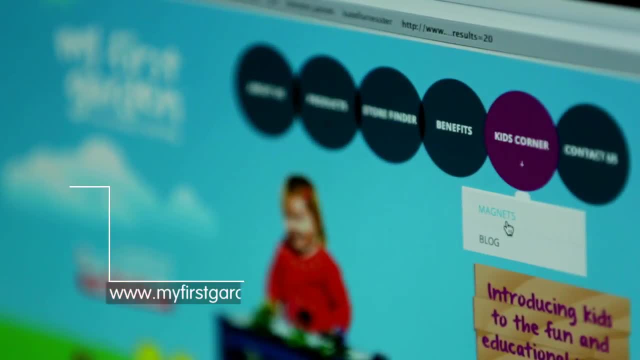 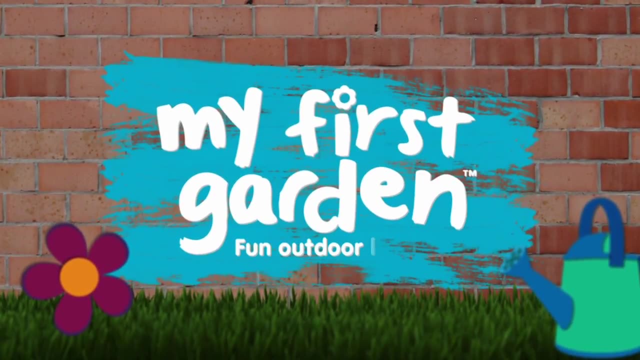 Plus, they can download templates from our website to make extra magnets which can be used to identify different plants, fruit and vegetables. My First Garden: Fun, outdoor learning.